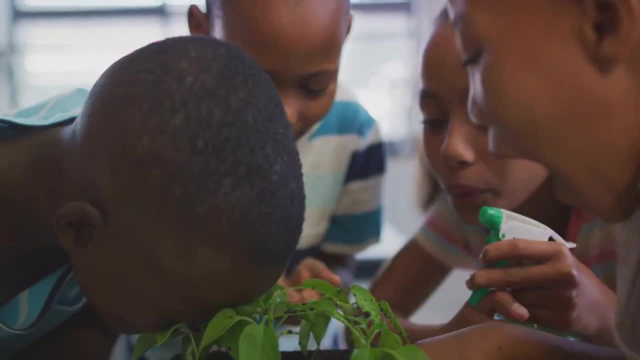 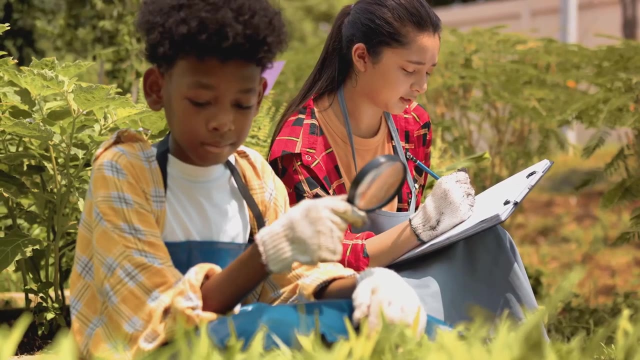 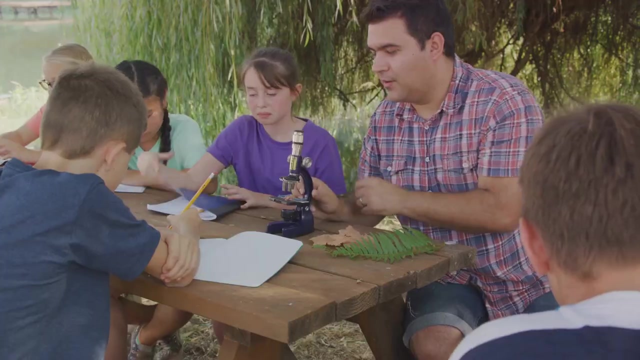 and fauna, fostering an understanding of the country's diverse ecosystems. These spaces are more than just gardens. They are vibrant classrooms under the open sky where the lessons are woven into the fabric of nature. Here children learn about life cycles as they watch a caterpillar. 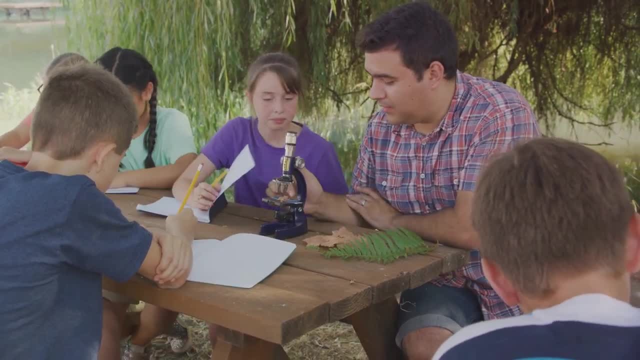 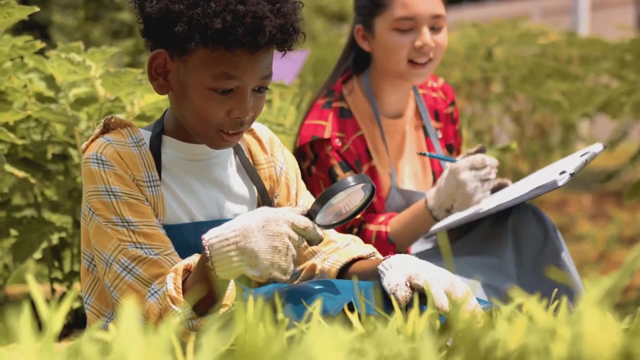 transform into a butterfly. They learn about the importance of pollinators as they observe bees flitting from flower to flower. They learn about patience and perseverance as they wait for their seeds to sprout and grow. A children's garden is a wonderland crafted for exploration. 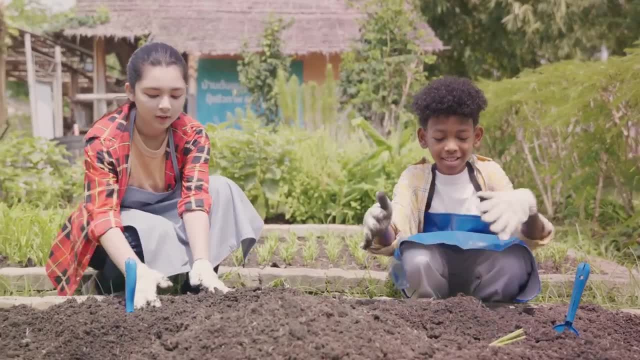 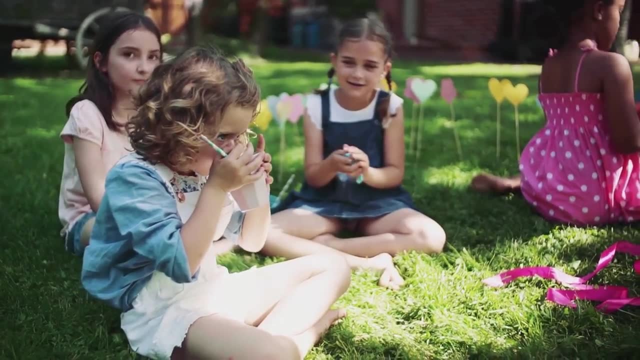 learning and growth. It's a place where every plant tells a story, every creature plays a part and every moment is an opportunity for discovery. Welcome to the vibrant world of children's gardens. Transforming a patch of earth, the children's garden is a place where they can explore the 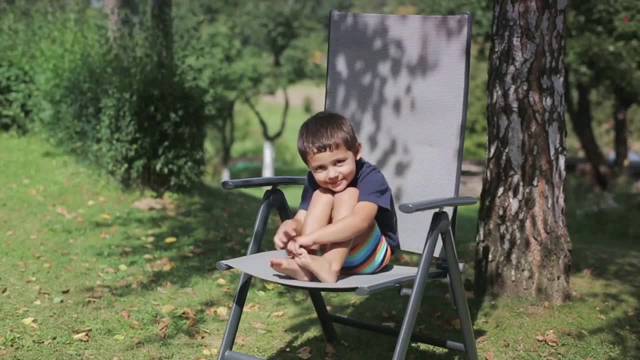 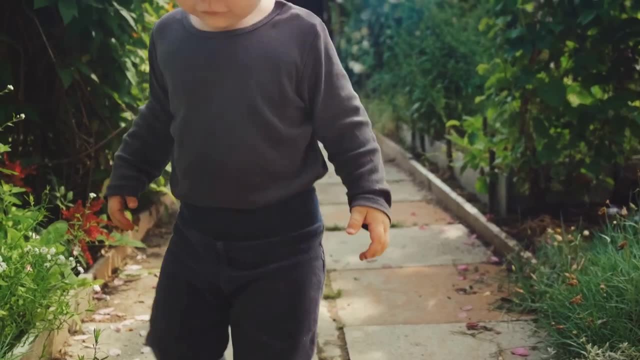 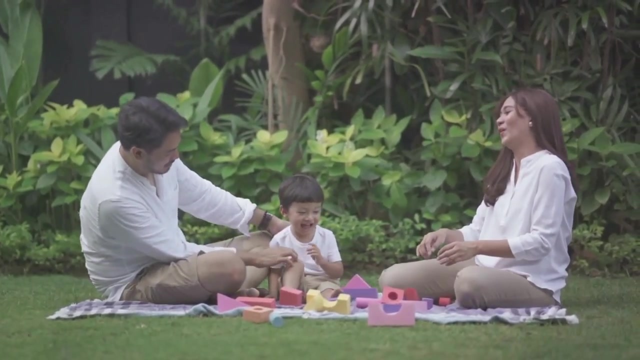 earth into a child's wonderland begins with imagination. The planning stage is your canvas, where you sketch out the pathways for exploration, the corners for discovery and the spaces for play. So how do we begin? First, selecting the right location is key. Consider an area that. 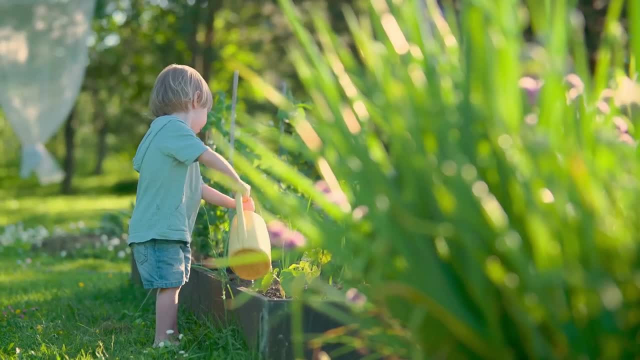 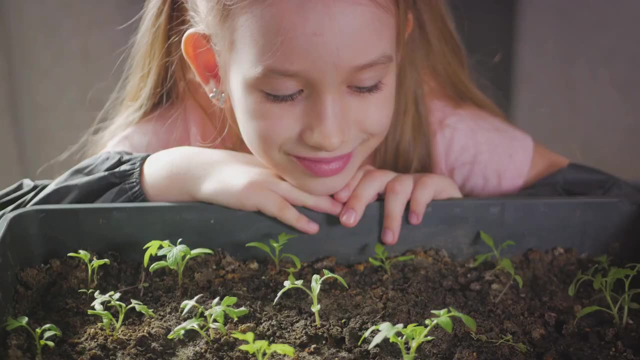 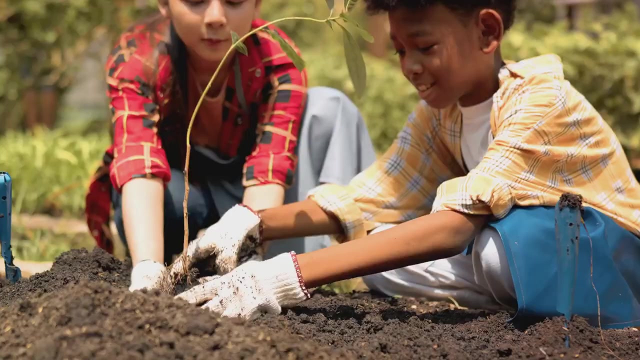 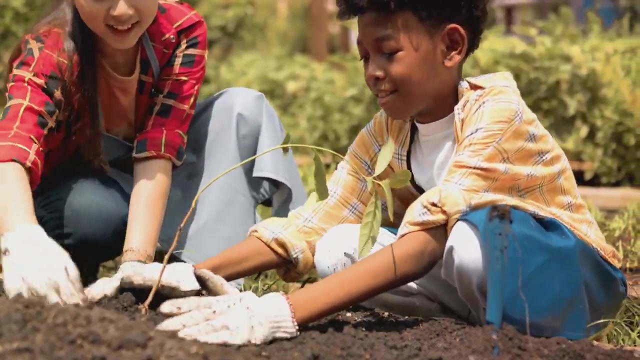 receives ample sunlight but also has some shade. This ensures that your garden is a comfortable place for children to play and learn, even in the height of summer. Next, it's time to choose your garden's place. Remember, this is a children's garden. Opt for plants that are safe and non-toxic, but also 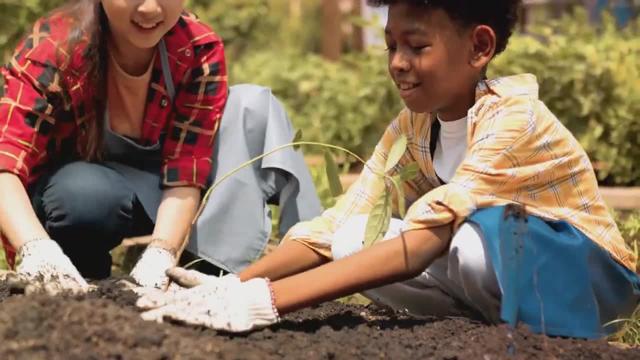 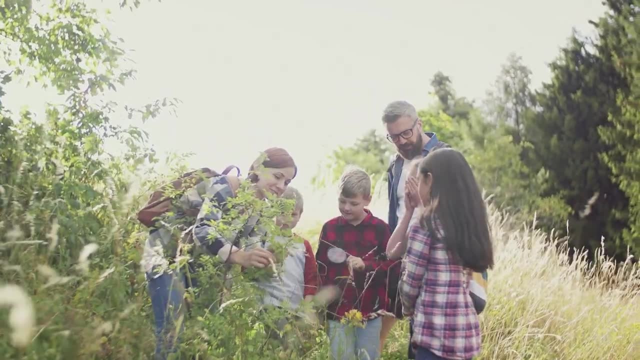 vibrant and engaging. Think sunflowers reaching for the sky, tomato plants heavy with bright red fruit and fragrant herbs like mint and lavender. These choices not only create a sensory feast for the little ones, but also offer opportunities for learning and discovery. Now let's talk about the 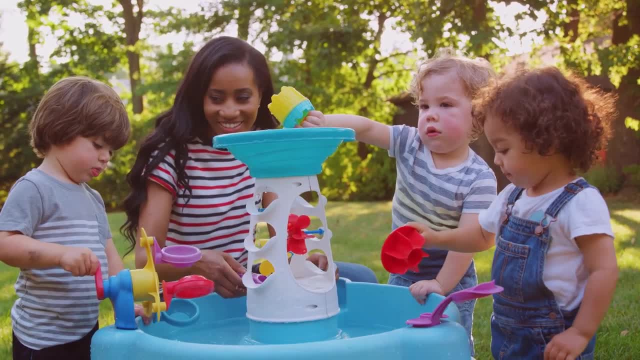 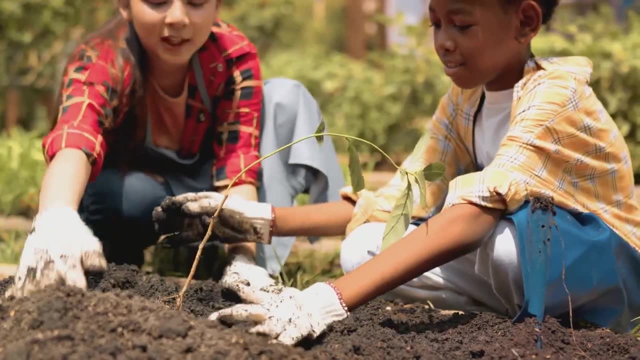 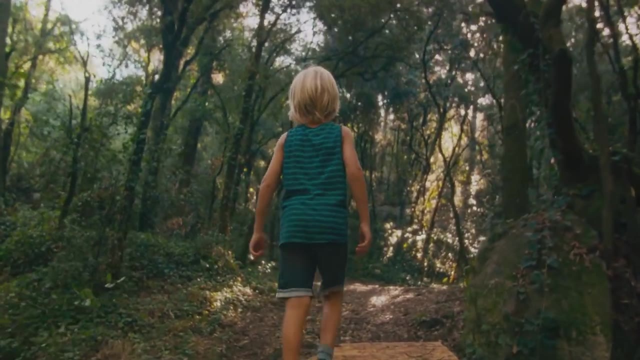 get their hands dirty. consider incorporating elements like a digging pit, a bird feeder or even a little pond. these features encourage children to engage with nature directly, fostering a sense of curiosity and wonder. don't forget the paths: meandering pathways invite exploration and add an element of adventure. use materials that are safe and comfortable. 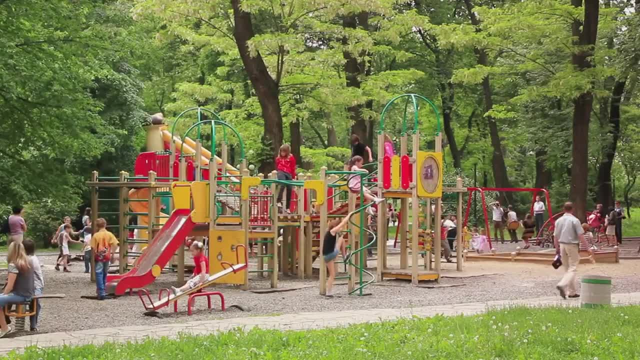 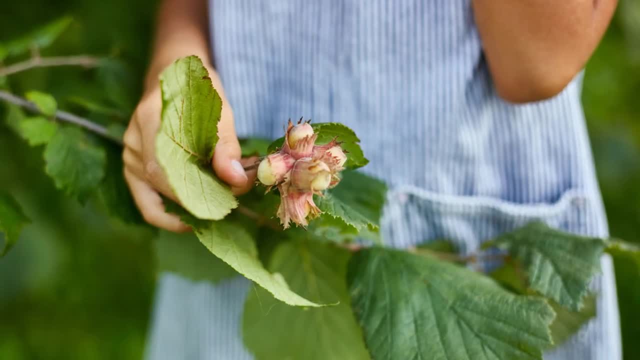 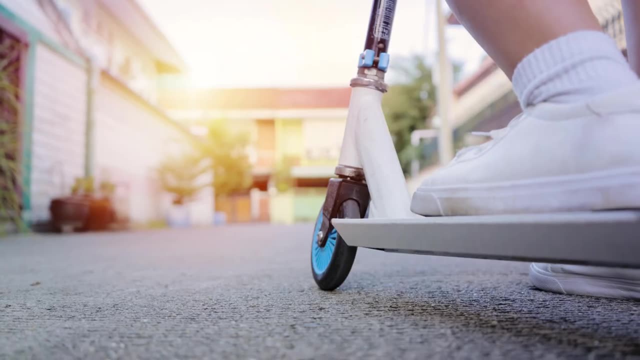 for little feet, like wood chips or smooth stones. lastly, consider adding some educational signage. simple, colorful signs can help children learn the names of plants, understand their life cycles and appreciate their importance in our ecosystem. remember, the goal is to create a space that's not just beautiful but also engaging and educational, a place where children can explore. 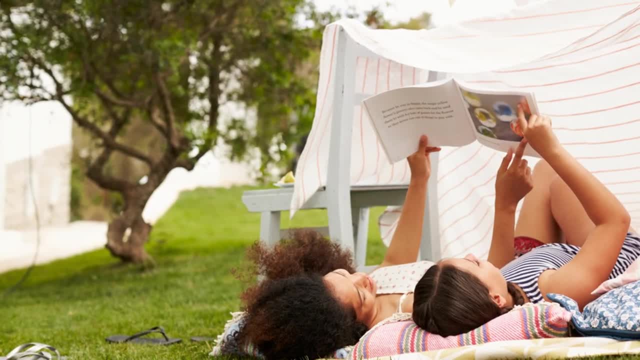 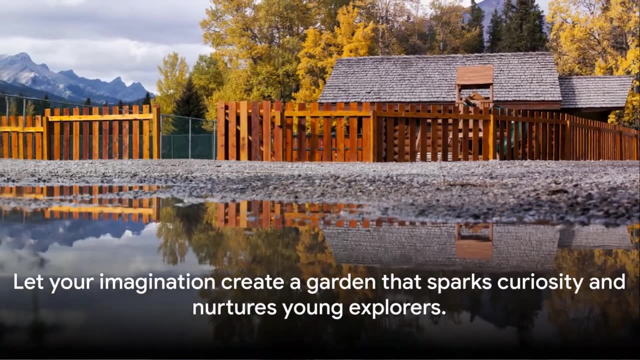 learn and grow. the planning stage is the foundation of your magical garden, where every choice becomes a part of a child's adventure. so let your imagination take the lead and create a wonderland that tells a story that will inspire you to explore and explore and explore and explore. 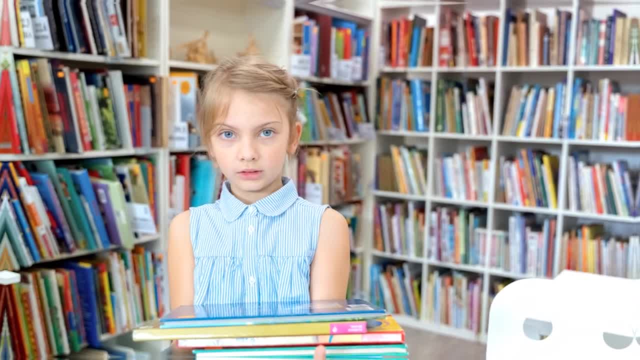 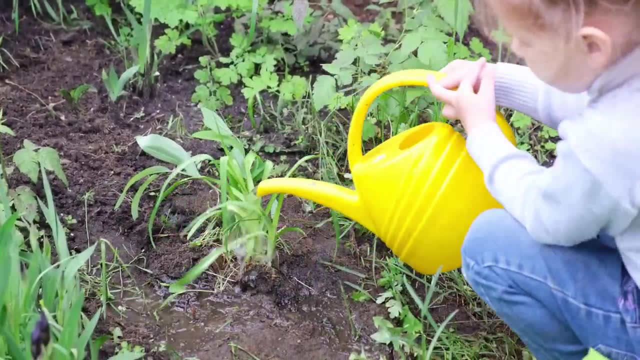 sparks curiosity and nurtures the little explorers in your life. from sowing a seed to watching it grow, each activity in a children's garden is an opportunity for hands-on learning and fun. imagine a child's thrill as they plant their first seed, the anticipation as they water. 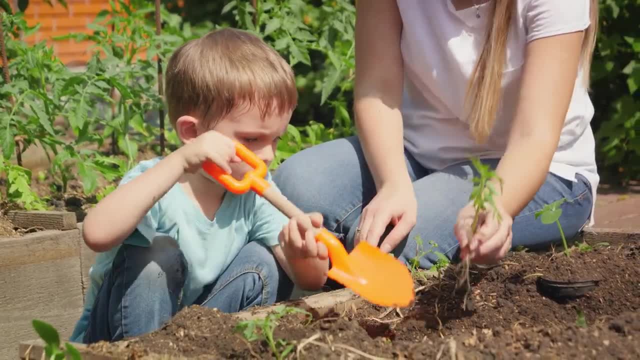 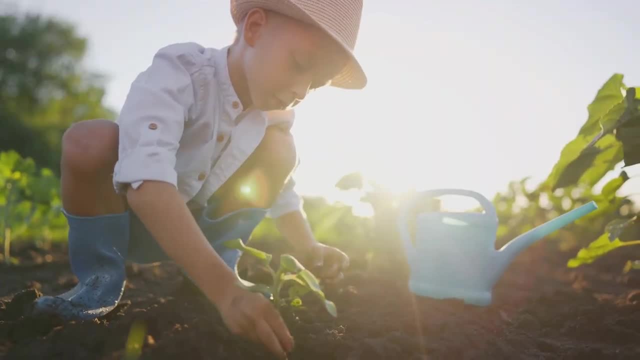 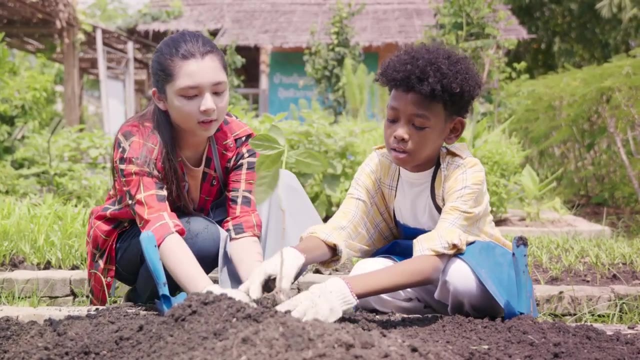 it: the excitement as they see the first sprout break through the soil, and the joy as they watch it grow into a vibrant plant. each of these stages is not just a gardening task but a lesson in life, growth and nature. gardening activities are full of learning opportunities that can spark curiosity. 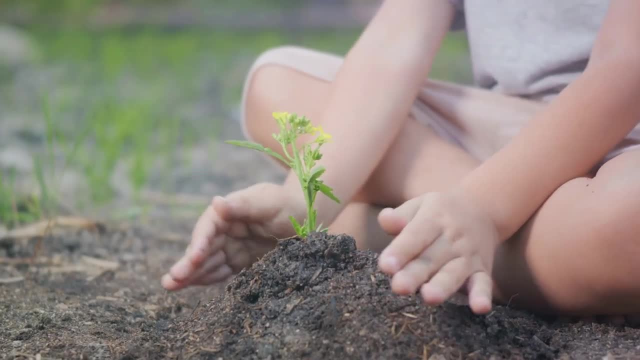 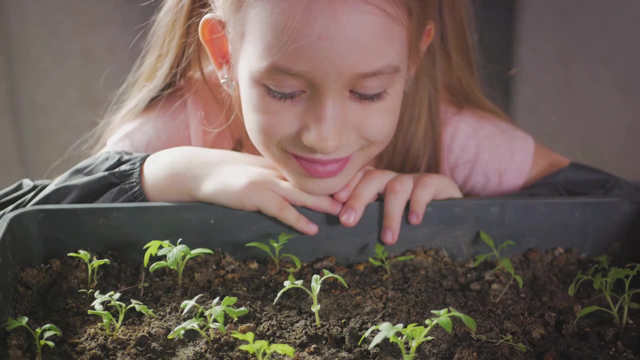 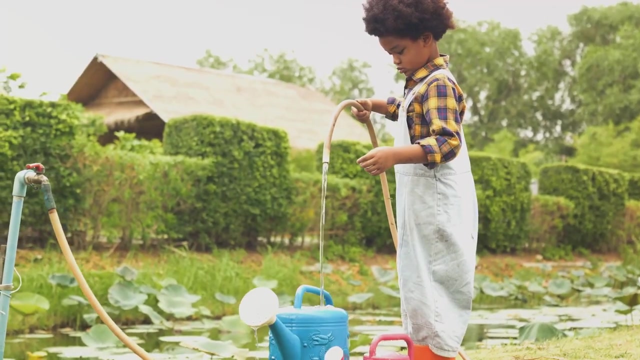 and foster a love for nature. planting seeds, for instance, can teach children about the life cycle of plants. they get to understand first hand how a tiny seed can grow into a beautiful flower or nutritious vegetable. it's a lesson in patience, care and the magic of life watering. 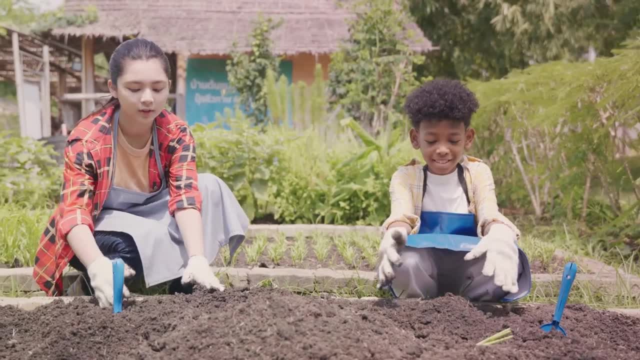 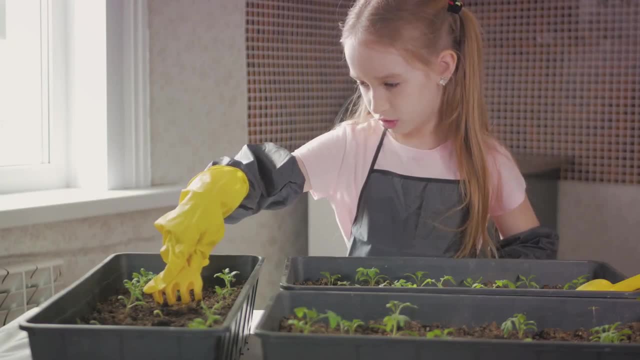 plants is another activity that's both fun and educational. StoryTalk videos, children's garden: everybody´s used to watching the flowers. Children learn about the importance of water for life and how proper care and attention can help living things thrive. It's not just about pouring water onto soil. it's about understanding the needs of living things and how to take care of them. 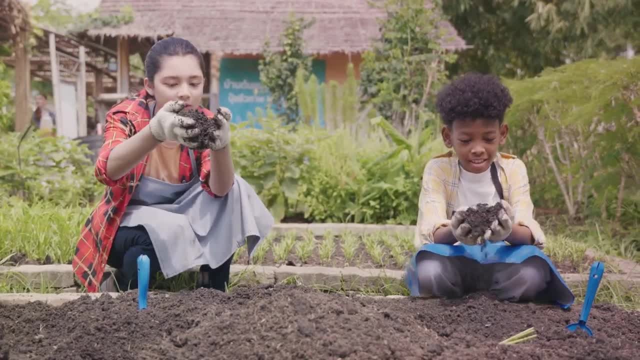 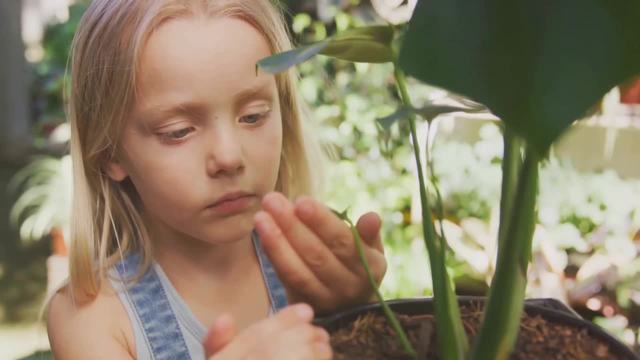 Exploring the garden can be a daily adventure. Each corner can reveal a new discovery, be it a sprouting seed, a blooming flower or a visiting insect. It's an open-ended exploration that can lead to countless questions and answers, sparking a sense of wonder and a thirst for knowledge. 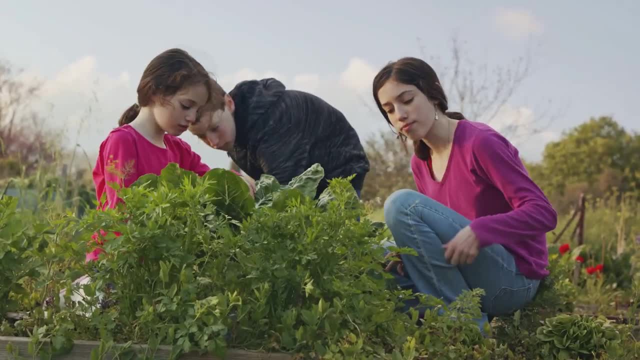 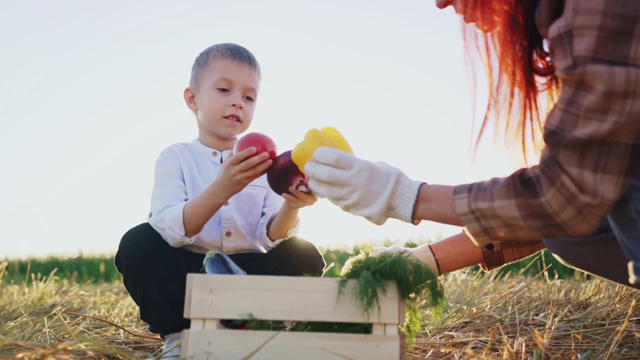 And then there's the joy of harvesting. After weeks of caring for their plants, children get to see the fruits of their labor, They learn about the rewards of patience and hard work, and they get to enjoy the fresh produce they've grown with their own hands. 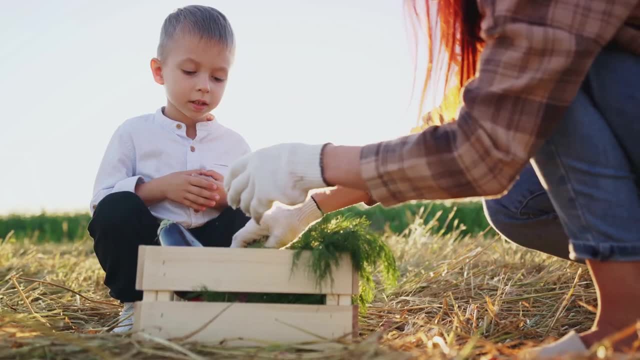 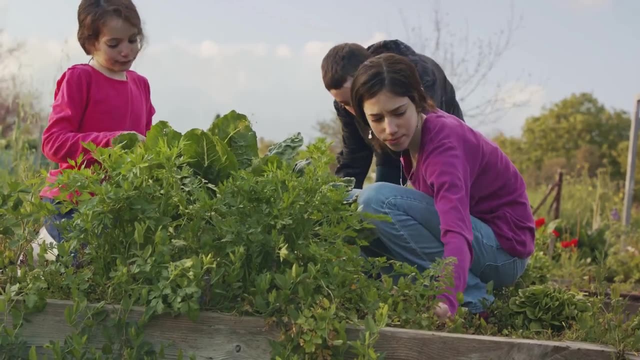 It's a delicious lesson in self-reliance and the cycle of nature. Each activity in the garden brings a new lesson, a new discovery And a new memory. So let's roll up our sleeves, dig into the soil and embark on a journey of fun and learning in the garden. 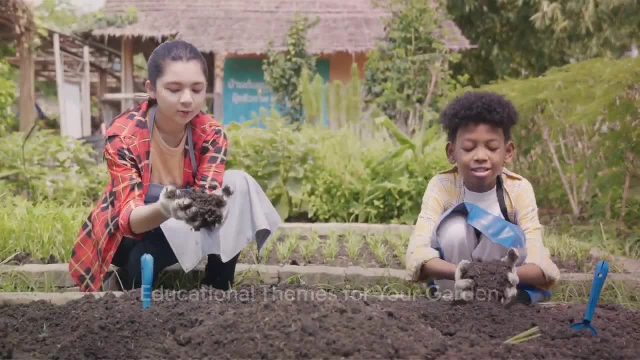 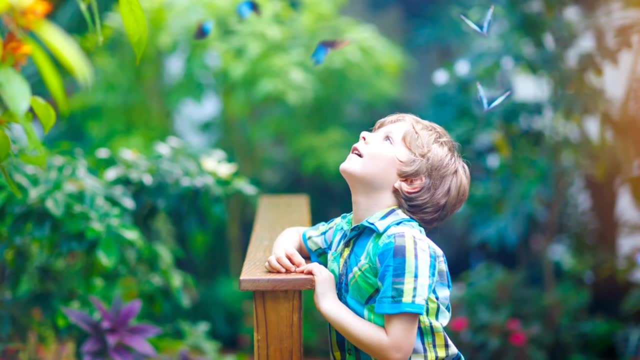 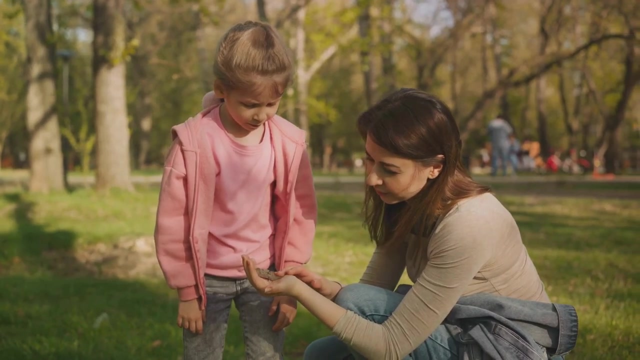 Transform your garden into an outdoor classroom with fascinating themes. The possibilities are as endless as your imagination and the curiosities of the children. One idea is to create a butterfly garden. With the right selection of plants like milkweed and butterfly bush, you can attract these winged jewels. 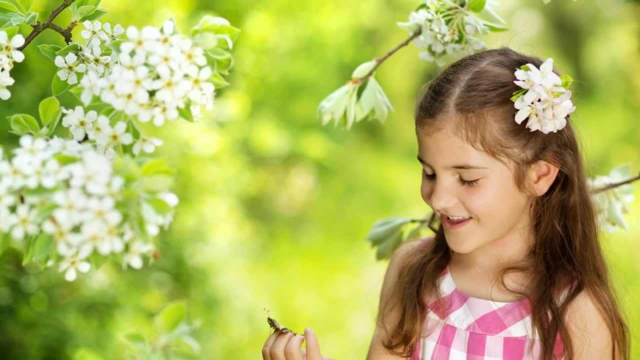 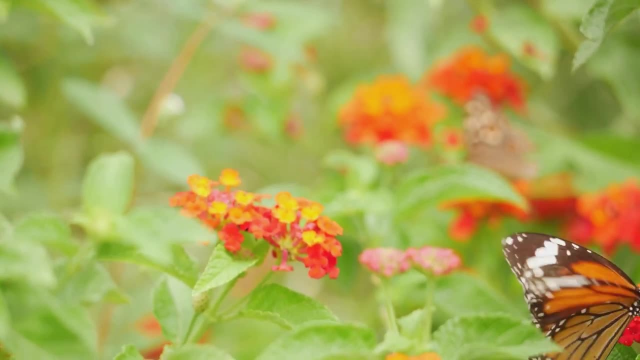 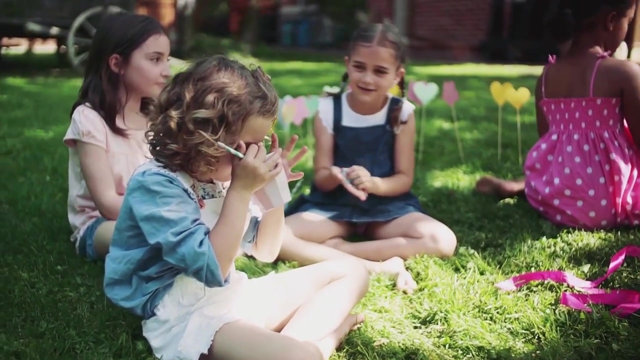 turning your garden into a living exhibit on the ground. Children will be captivated by the transformation from tiny eggs to caterpillars, chrysalises and, finally, beautiful butterflies. Another engaging idea is a sensory garden. This is a space designed to stimulate all five senses. 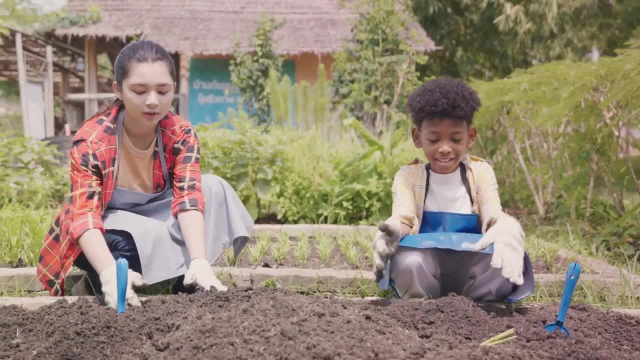 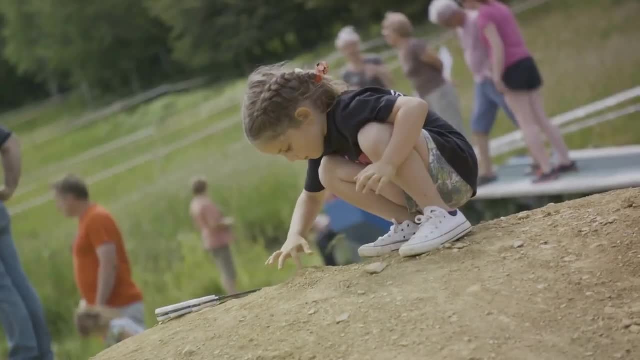 Think fuzzy lamb's ear for touch, fragrant lavender for smell, rustling bamboo for sound, kaleidoscopic flowers for sight, and edible herbs like mint for taste. A sensory garden can help children develop their sensory skills and appreciate the diversity of nature. 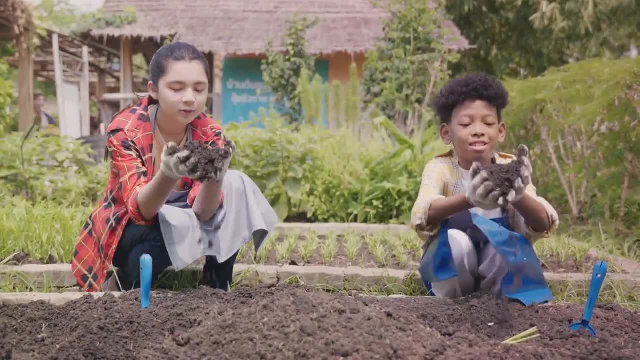 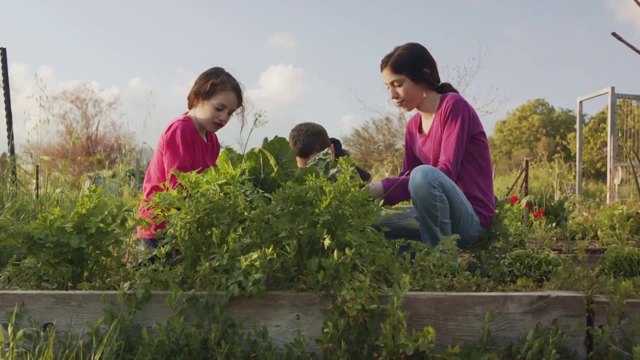 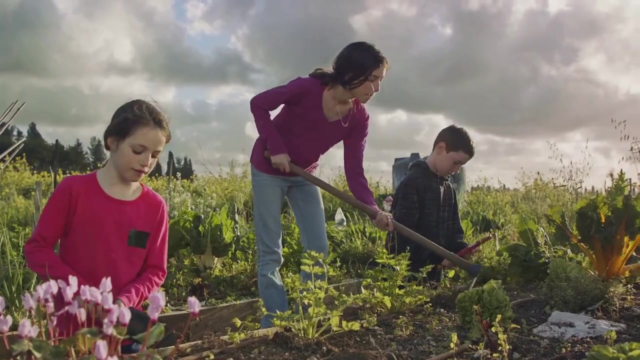 Don't forget about an edible garden. This can be a fun and practical way to teach children about where food comes from. They can plant, tend, harvest and even cook with the produce they've grown themselves. This hands-on experience can encourage healthier eating habits and foster a sense of responsibility. 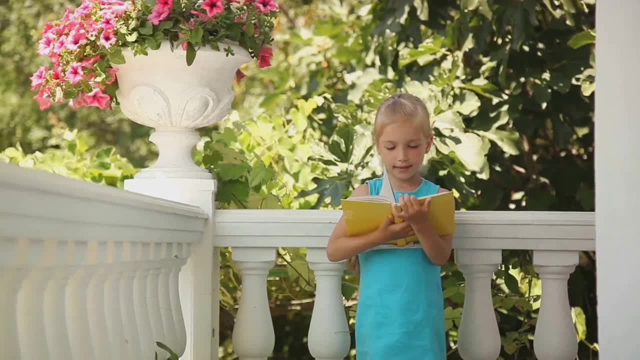 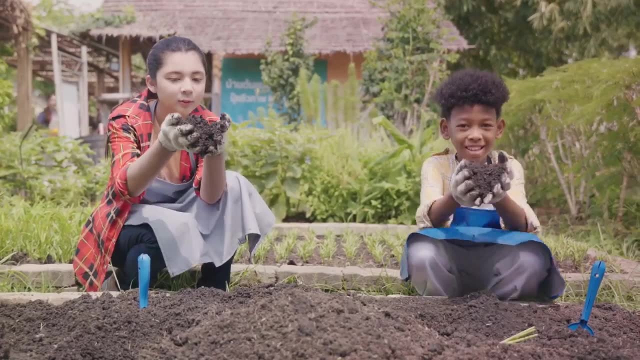 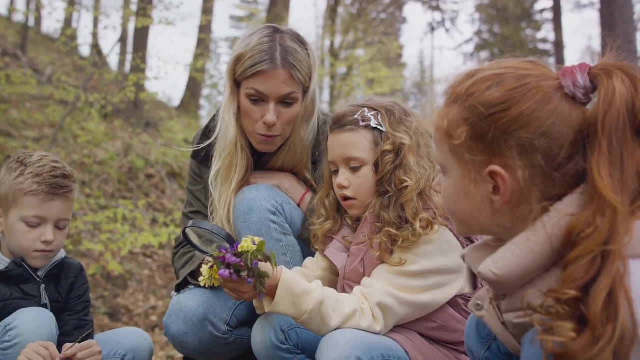 To make the most out of these themed areas, consider incorporating educational signage. This can be as simple as labeling plants and their uses, or as complex as explaining the processes of photosynthesis or pollination. Interactive activities like scavenger hunts or craft projects can also provide fun, practical lessons about nature, plants and ecosystems. 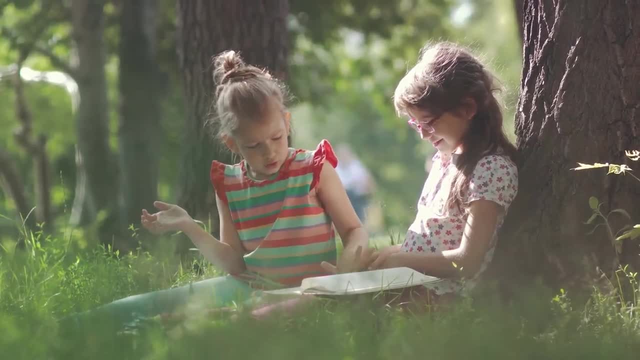 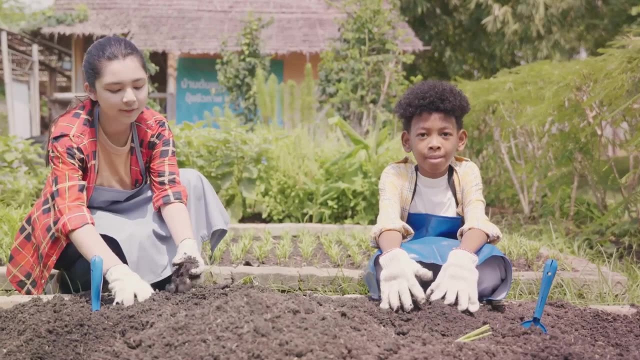 How about a storybook garden? Choose a favorite children's book and bring it to life through plants and garden features. This can inspire a love for literature and nature simultaneously. Remember the key to a successful educational garden is to keep it interactive, engaging and fun. 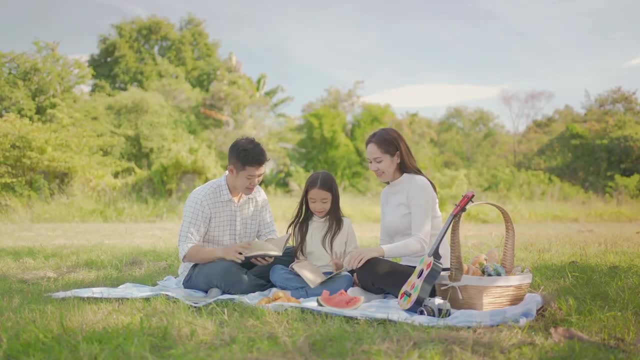 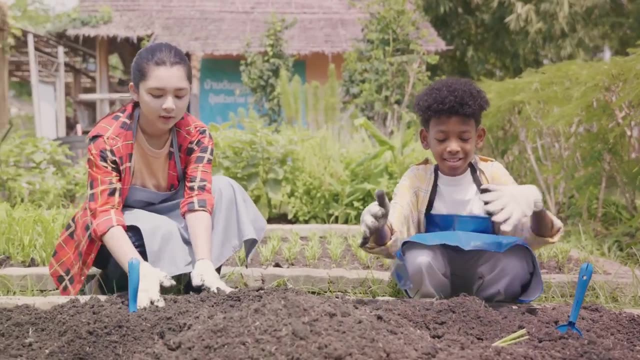 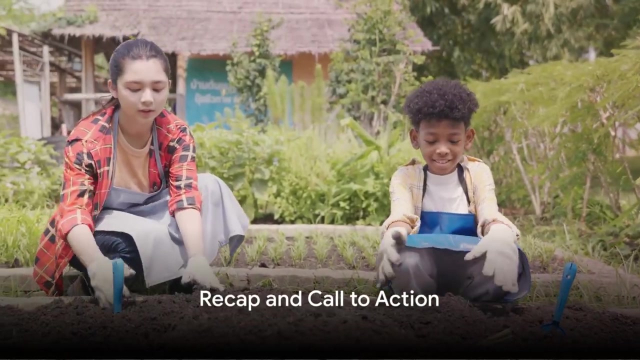 It's not about formal lessons or strict curriculums. It's about sparking curiosity, encouraging exploration and nurturing a love for nature. With the right themes, your garden can become a living classroom, turning every moment into a learning opportunity. Creating a children's garden is a journey of fun and education. 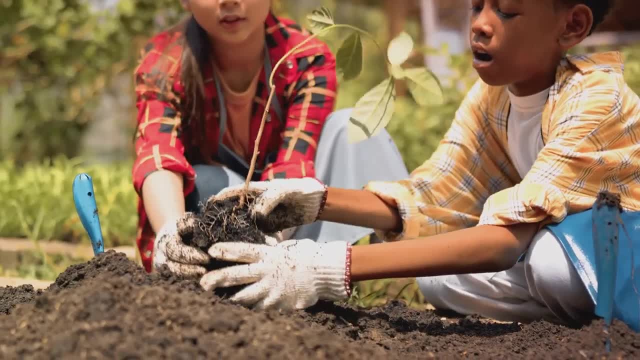 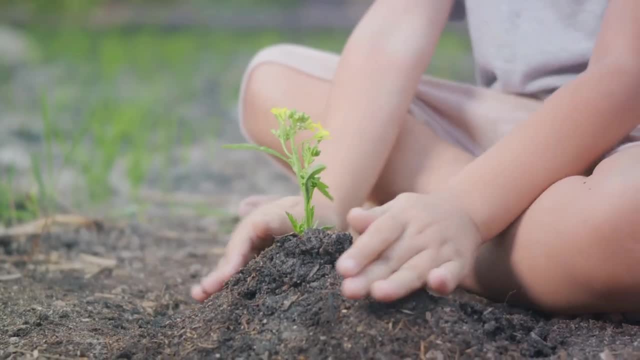 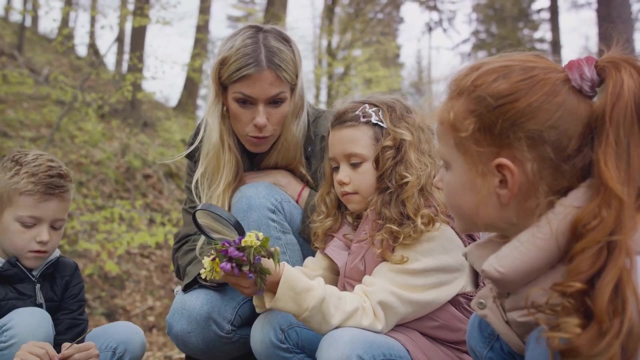 transforming tiny seeds into lifelong memories. We've taken a delightful stroll through the vibrant world of children's gardens, where every plant sparks curiosity and every corner tells a story. These magical wonderlands, crafted for exploration, learning and growth, give children a unique chance to connect with nature while having a blast. 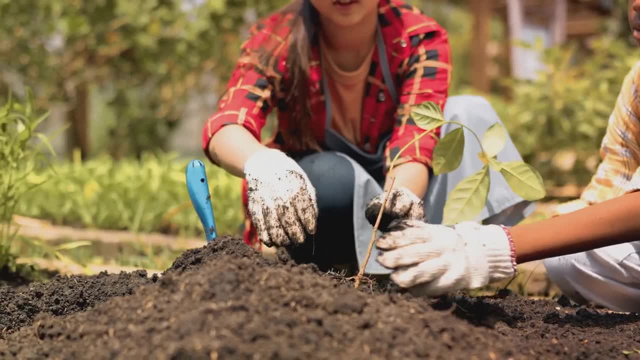 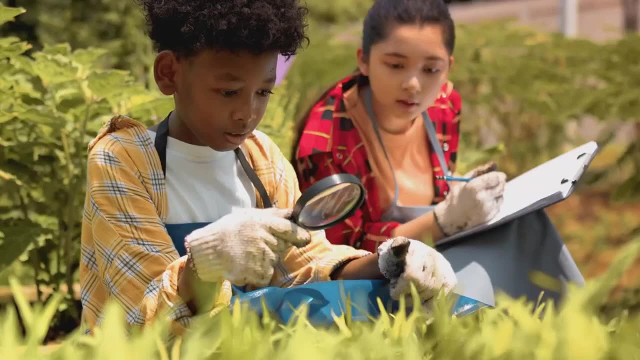 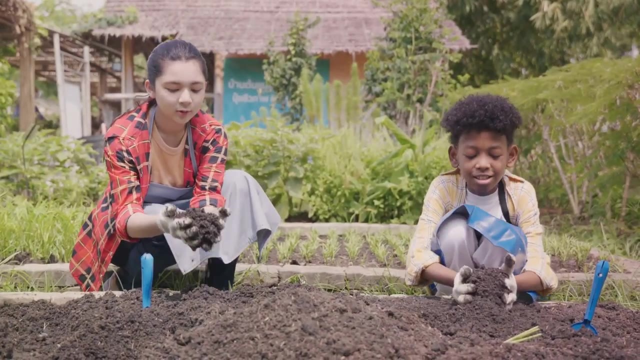 In planning your children's garden. we've learned the importance of imagination, from choosing vibrant, safe plants to interactive elements that engage all the senses. Remember, the goal is to create a space that encourages hands-on learning and discovery. We've also delved into the wide array of engaging activities that can take place in the garden. 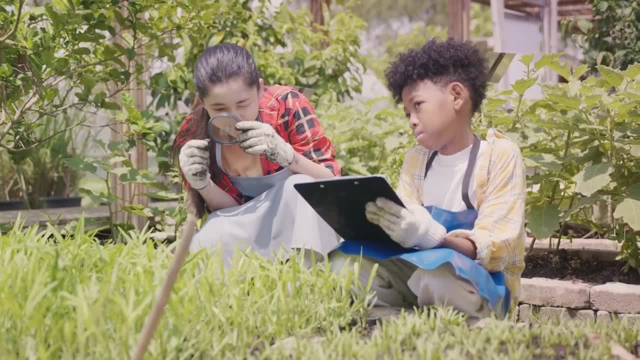 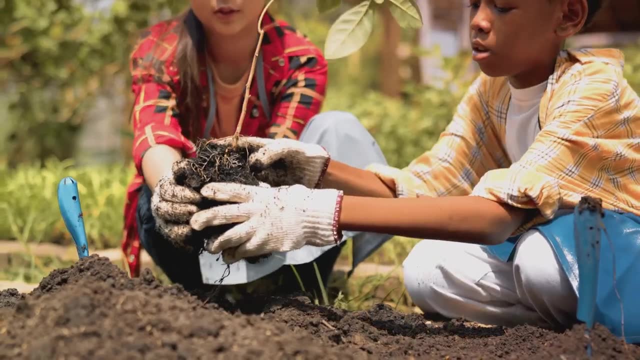 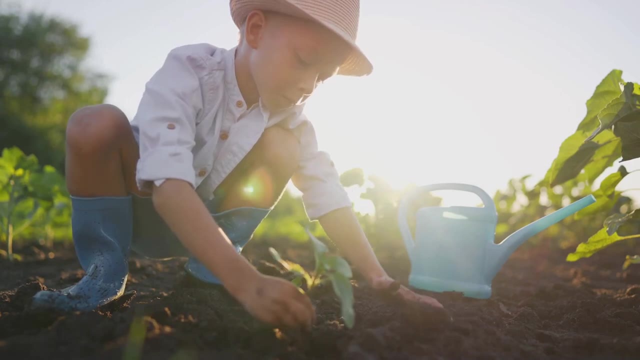 each one an opportunity for hands-on learning and fun, From seed planting to vegetable harvesting. these activities not only teach children about the natural world, but also instill a sense of responsibility and achievement. Then we explored the power of educational themes to transform your garden into a living classroom. 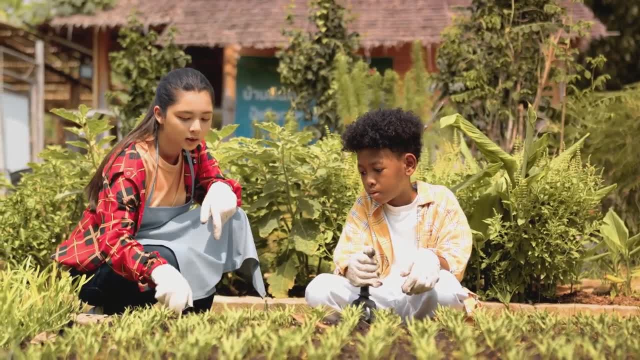 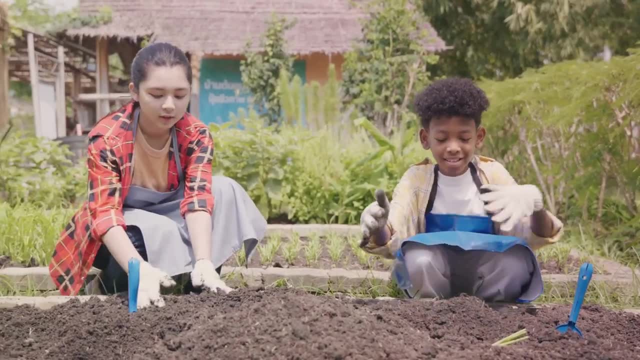 Whether it's a butterfly garden, a sensory garden or a vegetable plot, these themes fascinate and educate, turning little moments into big discoveries. But remember the journey to create a children's garden doesn't end with the last plant in the ground. 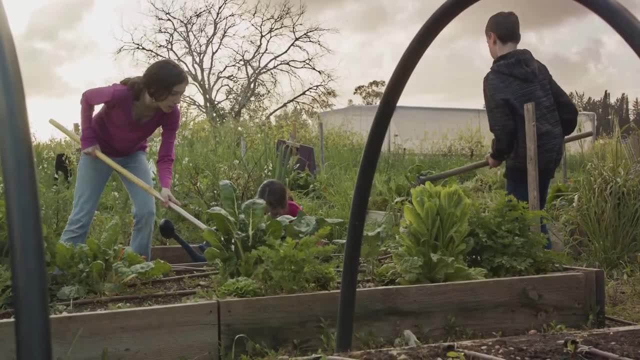 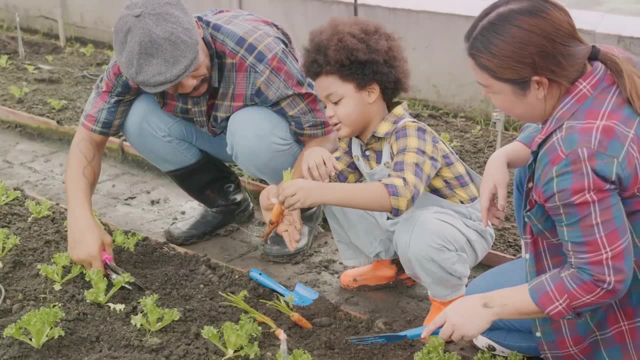 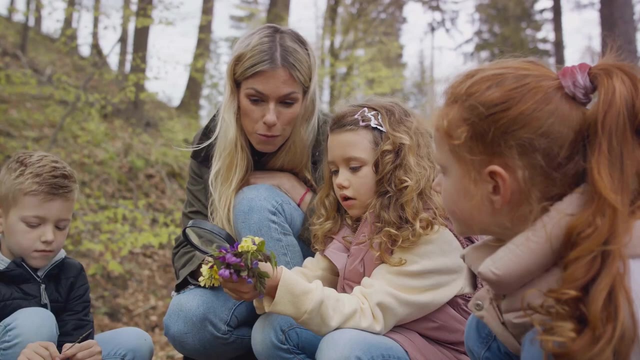 This adventure continues as the garden grows and evolves, just like the children who tend it. Share your journey, inspire others and create a community of garden enthusiasts. So why not get started on your own children's garden today? Let the magic of nature captivate the young minds in your life. 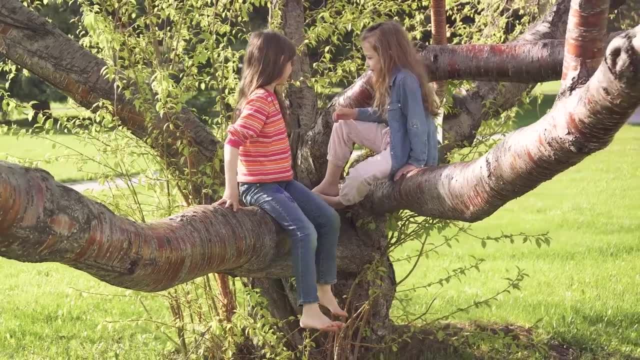 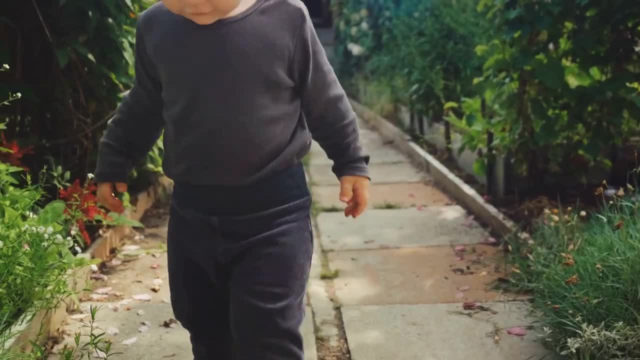 Encourage their curiosity, foster their love for the outdoors and watch as they grow, just like the seeds they plant. Embark on this delightful journey to create a children's garden. Share your story, inspire others and watch as tiny seeds grow into lifelong memories.